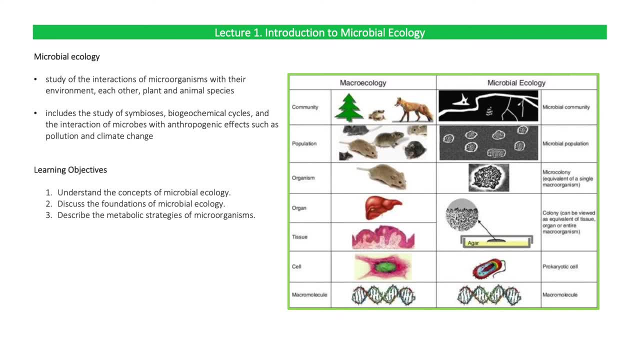 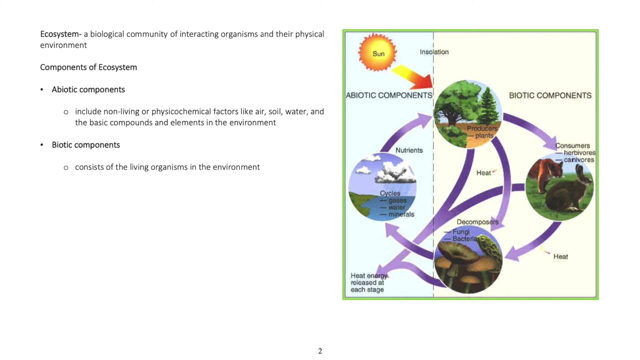 Learning Objectives: 1. Understand the concepts of microbial ecology. 2. Discuss the foundations of microbial ecology. 3. Describe the metabolic strategies of microorganisms. Ecosystem: A biological community of interacting organisms and their physical environment. Components of Ecosystem: Abiotic Components Include non-living or psychochemical factors like air, soil, water and the basic compounds and elements in the environment. 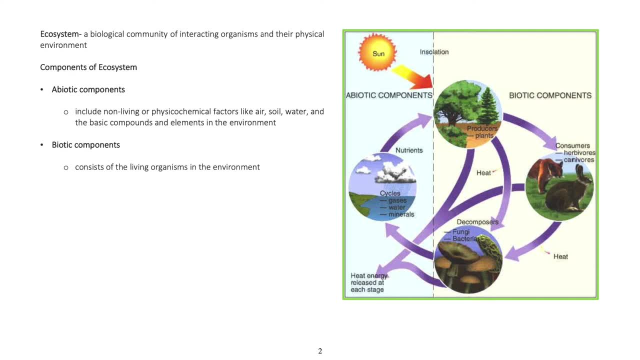 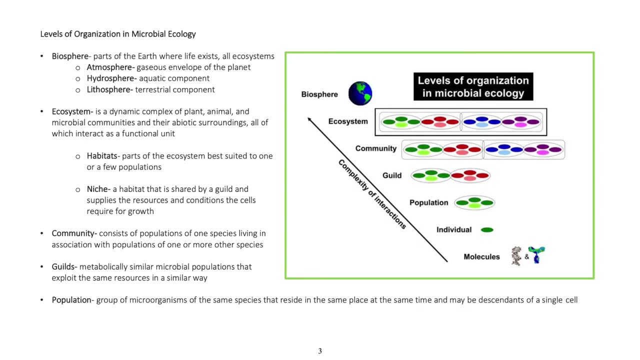 Biotic Components Consists of the living organisms in the environment, Levels of Organization in Microbial Ecology, Biosphere, Parts of the Earth where life exists, all ecosystems, Ecosystems, Atmosphere, Gaseous Envelope of the Planet, Hydrosphere. Aquatic Component. 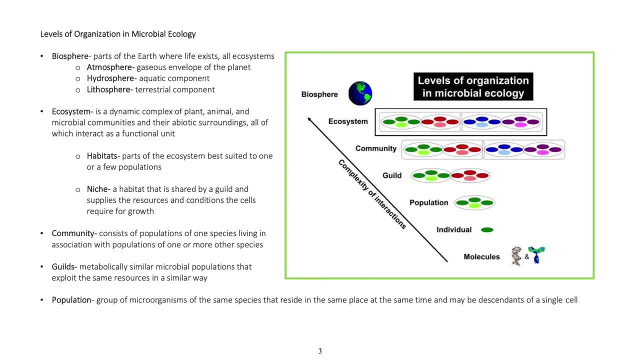 Lithosphere Terrestrial Component. Ecosystem Is a dynamic complex of plant, animal and microbial communities and their abiotic surroundings, all of which interact as a functional unit: Habitats, Parts of the Ecosystem, Ecosystem best suited to one or a few populations. 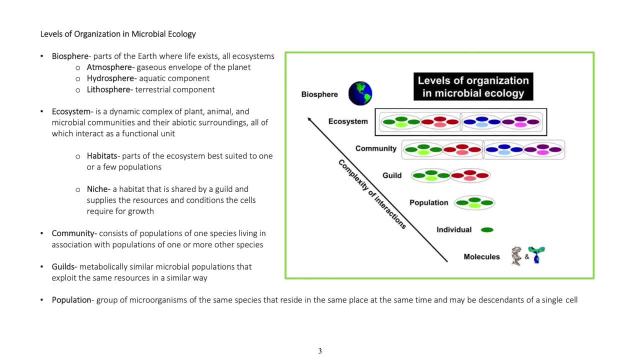 Niche: A habitat that is shared by a guild and supplies the resources and conditions the cells require for growth. Community Consists of populations of one species living in association with populations of one or more other species: Guilds, Metabolically similar microbial populations that exploit the same resources in a similar way. 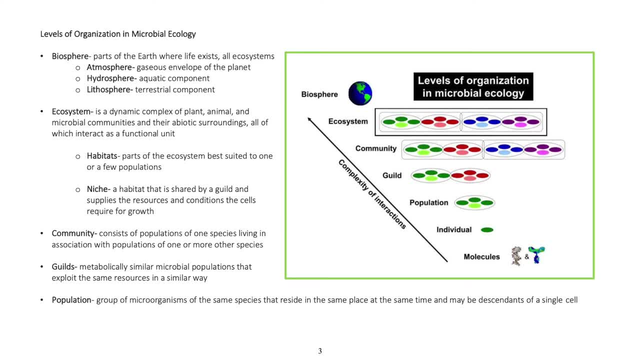 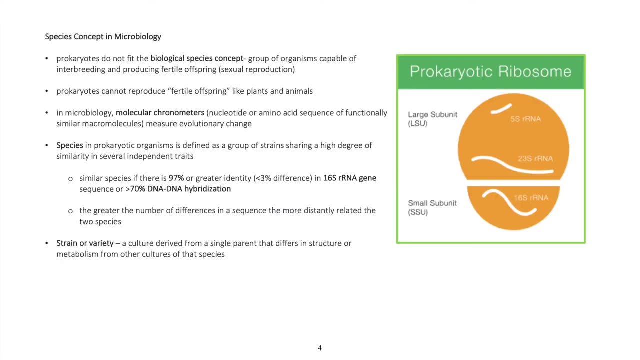 Ecosystems, Ecosystems, Christmas Microbiology- 보는 Species, Propaganda, The Douglas Items: sexual reproduction. Prokaryotes cannot reproduce fertile offspring like plants and animals. In microbiology, molecular chronometers of functionally similar macromolecules measure evolutionary change. Species in prokaryotic organisms is. 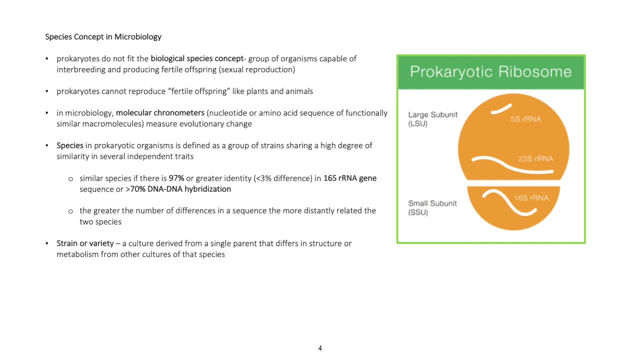 defined as a group of strains sharing a high degree of similarity in several independent traits. Similar species: If there is 97% or greater identity. less than 3% difference in 16S rRNA gene sequence or greater than 70% DNA-DNA hybridization, the greater the 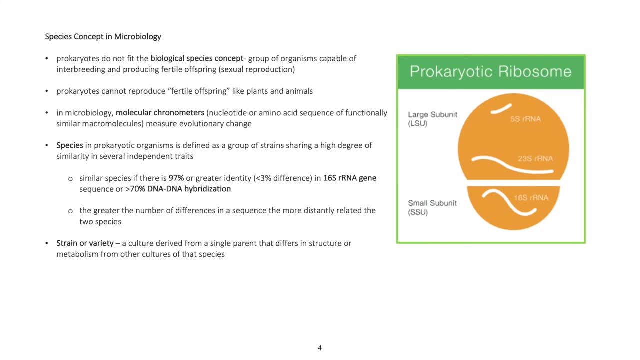 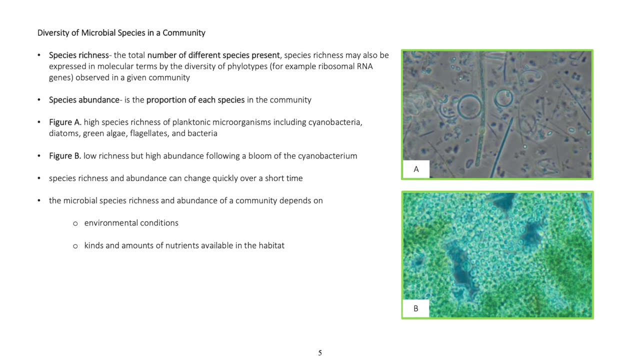 number of differences in a sequence: the more distantly related the two species. Strain or variety: A culture derived from a single parent that differs in structure or material Metabolism from other cultures of that species. Diversity of microbial species in a community: Species richness: The total number of different. 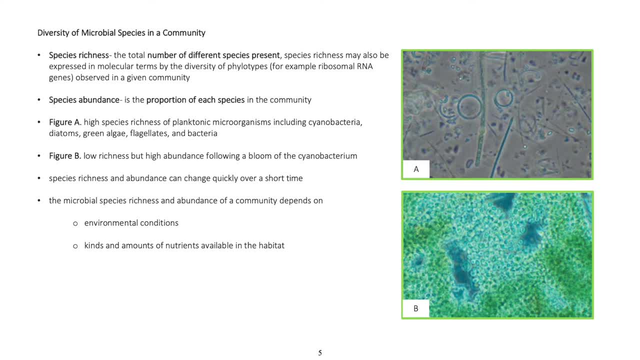 species present. Species richness may also be expressed in molecular terms by the diversity of phylotypes, For example ribosomal RNA genes, observed in a given community. Species richness Is the proportion of each species in the community. Figure A: High species richness of planktonic microorganisms, Including cyanobacteria diatoms. 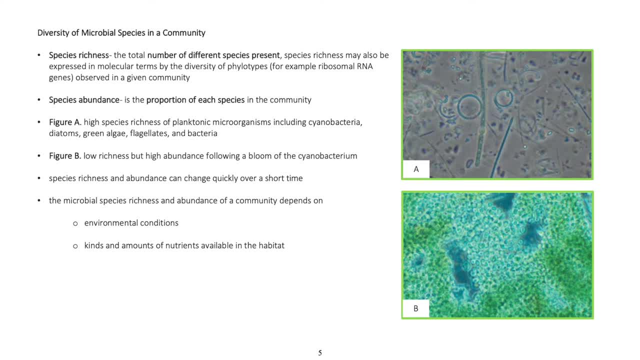 green algae, phylatulates and bacteria. Figure B- Low richness but high abundance following a bloom of the cyanobacterium Species, richness and abundance can change quickly over a short time. Figure C- High abundance following a bloom of cyanobacterium Species, richness and abundance can change. 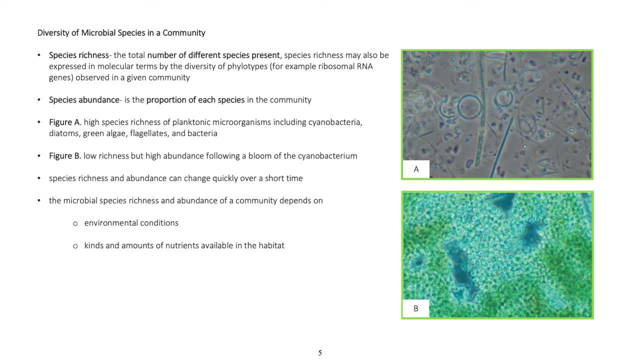 quickly over a short time. Figure D: High abundance following a bloom of the cyanobacterium. The microbial species, richness and abundance of a community depends on environmental conditions, kinds and amounts of nutrients available in the habitat. Martinus Bajerink. 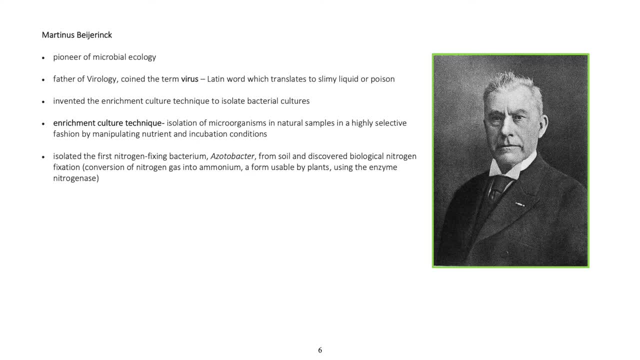 Pioneer of Microbial Ecology, Father of Virology, coined the term virus, Latin word which translates to slimy liquid or poison- Invented the enrichment culture technique to isolate bacterial cultures. Enrichment Culture Technique: Isolation of microorganisms in natural samples in a highly selected fashion, by manipulating nutrient and incubation conditions. 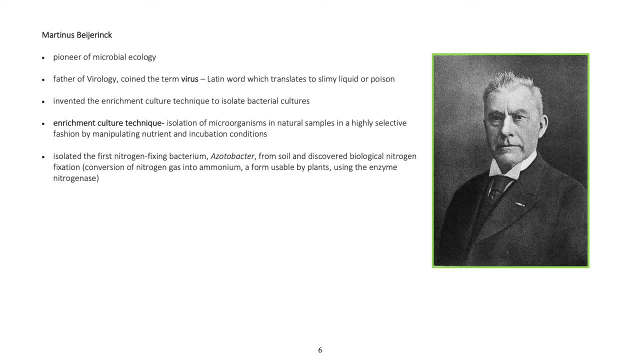 Isolated the first nitrogen fixing bacterium, Ozetobacter, from soil and discovered biological nitrogen fixation. Conversion of Nitrogen: Conversion of nitrogen gas into ammonium, a form usable by plants, using the enzyme nitrogenase Enrichment Culture. 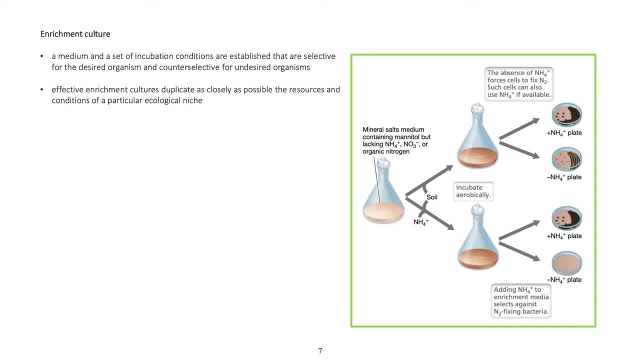 A medium and a set of incubation conditions are established that are selected for the desired organism and counter-selected for undesired organisms. Effective enrichment cultures duplicate as closely as possible the resources and conditions of a particular ecological nature. 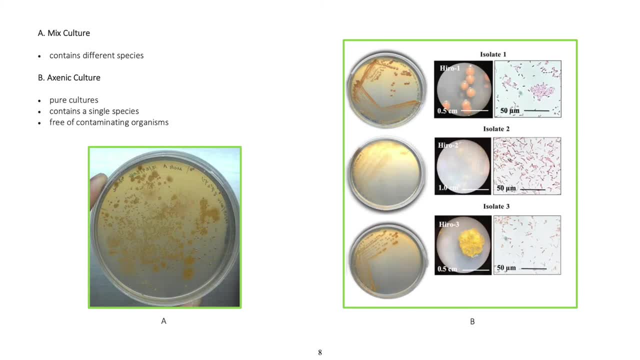 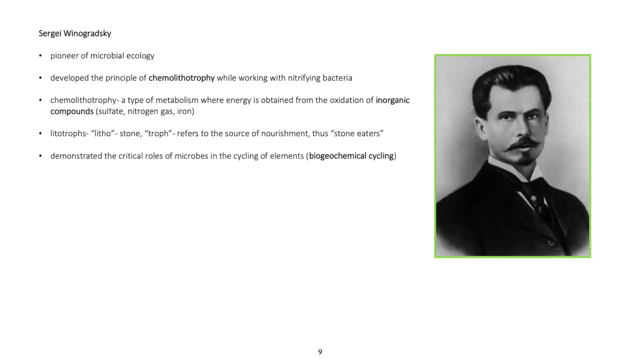 Niche, Mixed Culture Contains different species. Oxnick Culture- Pure Cultures- Contains a single species, Free of contaminating organisms. Sergei Winogradsky, Pioneer of Microbial Ecology, Developed the principle of chemolithotrophy. Chemolithotrophy: A type of metabolism. 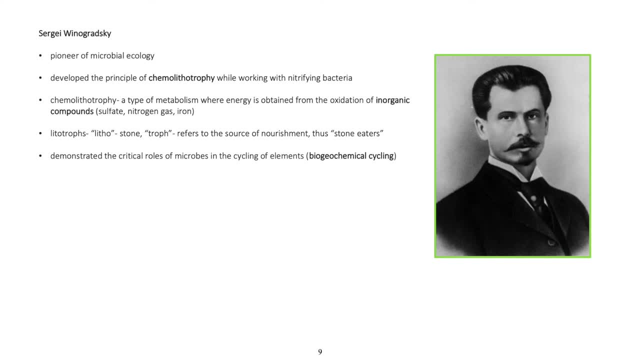 Where energy is obtained from the oxidation of inorganic compounds. Examples are sulfate, nitrogen gas and iron Lidotrophs. Litho- translates to stone and troph- refers to the source of nourishment. Thus, stone heaters demonstrated the critical roles of microbes in the cycling of elements or biogeochemical cycling. 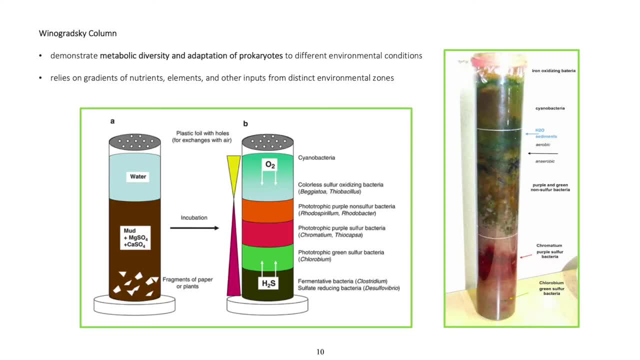 Winogradsky Column In the cycle of elements or biogeochemical cycling. Winogradsky Column Demonstrate metabolic diversity and adaptation of prokaryotes to different environmental conditions Relies on gradients of nutrients, elements and other inputs from distinct environmental zones. 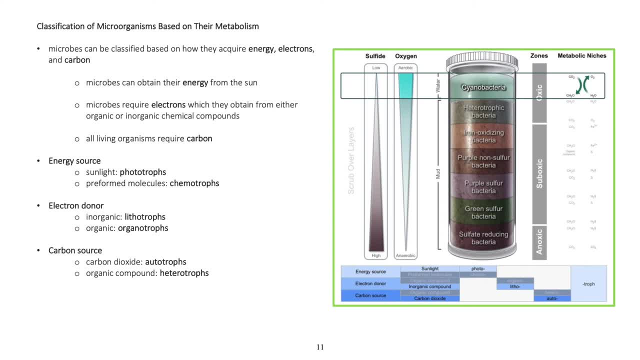 Classification of Microorganisms Based on Their Metabolism. Microbes can be classified based on how they acquire energy, electrons and carbon. Microbes can obtain a certain amount of energy, electrons and carbon. Microbes can obtain a certain amount of energy, electrons and carbon. 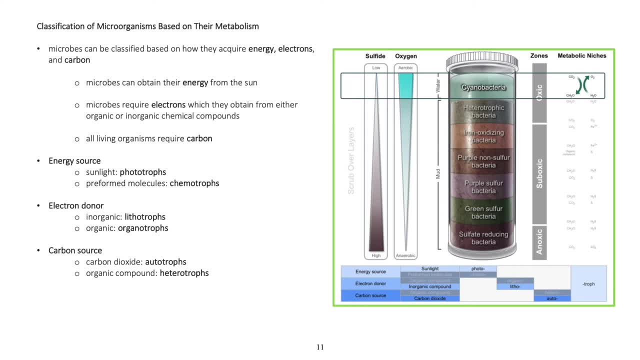 their energy from the sun, Microbes require electrons, which they obtain from either organic or inorganic chemical compounds. All living organisms require carbon energy source: sunlight, phototrophs, preformed molecules, chemotrophs, electron donor- inorganic. 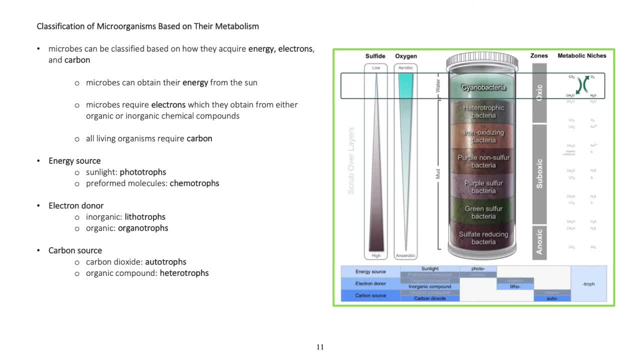 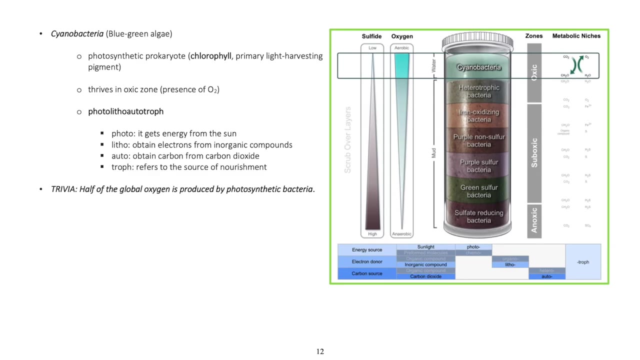 lithotrophs. organic organotrophs. carbon source, carbon dioxide. autotrophs organic compound heterotrophs. cyanobacteria, blue-green algae, photosynthetic prokaryote. presence of chlorophyll: primary light harvesting pigment thrives in oxyxone. 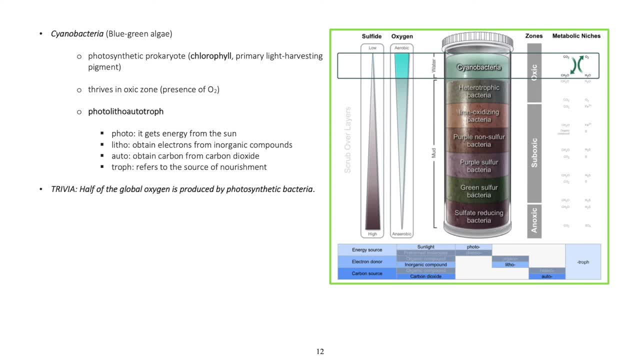 Presence of oxygen. Photolithotroph Photo. It gets energy from the sun. Litho Obtain electrons from inorganic compounds. Auto Obtain carbon from carbon dioxide. Troph Refers to the source of nourishment Trivia: Half of the global oxygen is produced by photosynthetic. 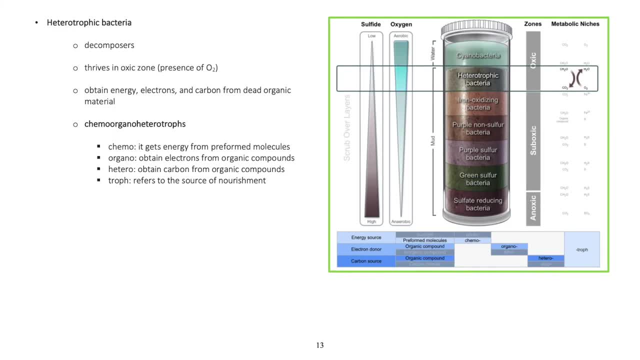 bacteria. Heterotrophic bacteria Decomposers, Thrives in oxyxone Presence of oxygen, Obtain energy, electrons and carbon from dead organic material. Chemo-organo-heterotrophs- Chemo- It gets energy. 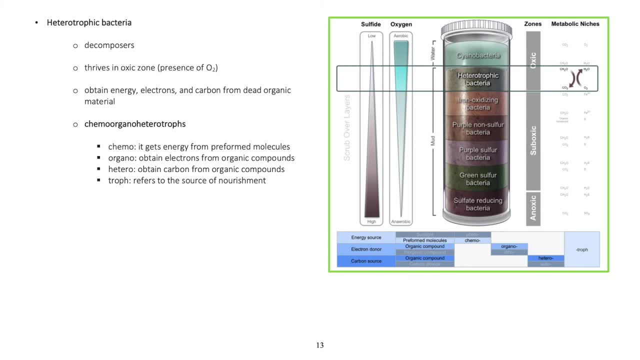 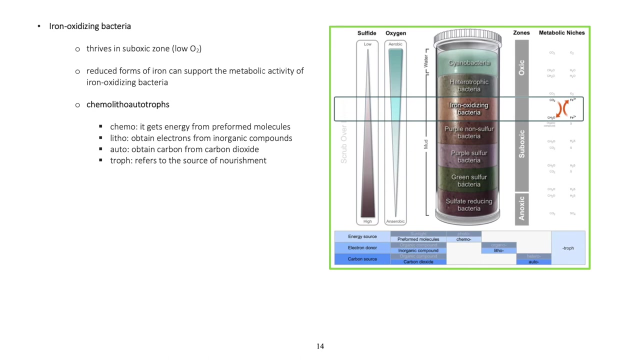 from preformed molecules. Organo Obtain electrons from organic compounds. Heterotrophs Obtain carbon from organic compounds. Troph Refers to the source of nourishment. Iron-oxidizing bacteria Thrives in suboxyxone with low oxygen. Reduced forms of iron can. 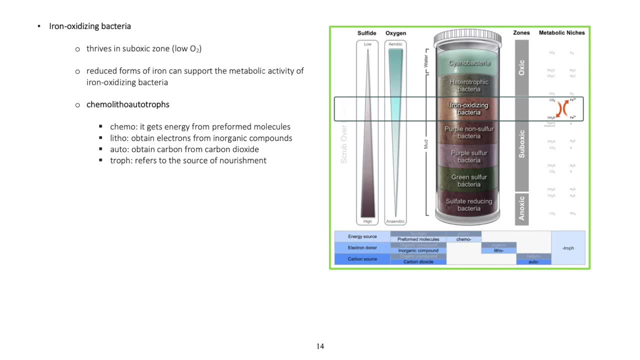 support the metabolic activity of iron-oxidizing bacteria, Chemolithotrophs. Chemo: It gets energy from preformed molecules. Litho: Obtain electrons from inorganic compounds. Auto Obtain electrons from inorganic compoundsины. 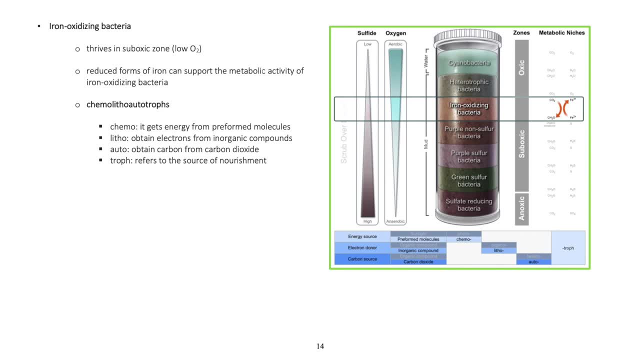 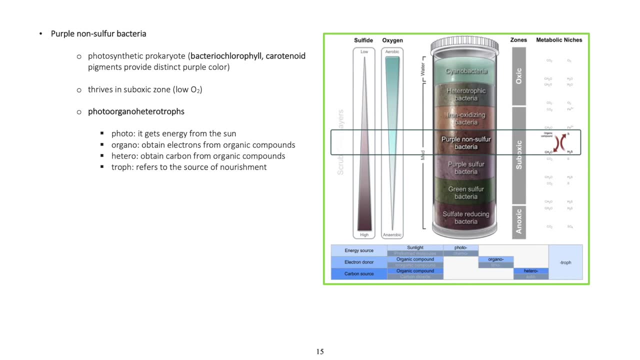 Oxide Troph Refers to the source of nourishment. Purple non-sulfur bacteria, Photosynthetic prokaryotes, Presence of bacterioclorophyll And carotenoid pigments which provide distinct purple color, Thrives in suboxic zone. low oxygen Photorgana and erotrophs Photo It. 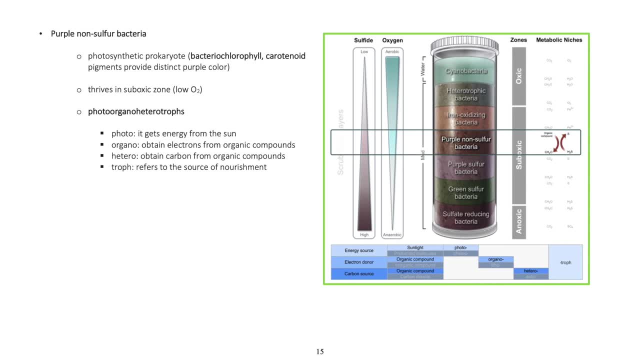 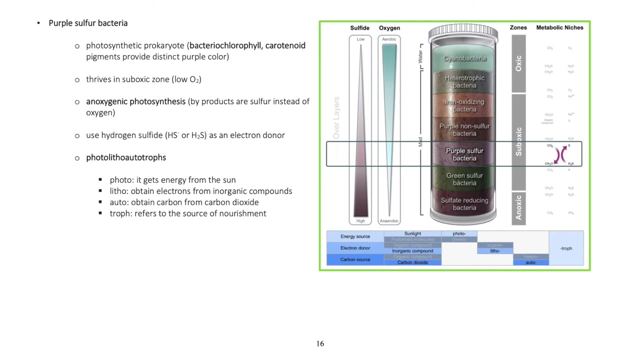 gets energy from the sun. Organo- Obtain electrons from organic compounds. Hetero- Obtain carbon from organic compounds. Troph Refers to the source of nourishment: Purple sulfur bacteria, Photosynthetic prokaryote. Presence of bacterioclorophyll And carotenoid pigments, which provide distinct 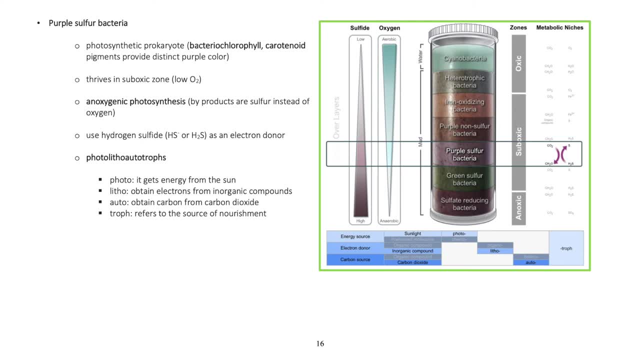 purple color Thrives in suboxic zone with low oxygen. Anoxygenic photosynthesis Byproducts are sulfur instead of oxygen. Use hydrogen sulfide as an electron donor. Photolithonidrophs Photo- It gets energy from the sun. Litho Obtain electrons from inorganic compounds. Auto Obtain carbon from. 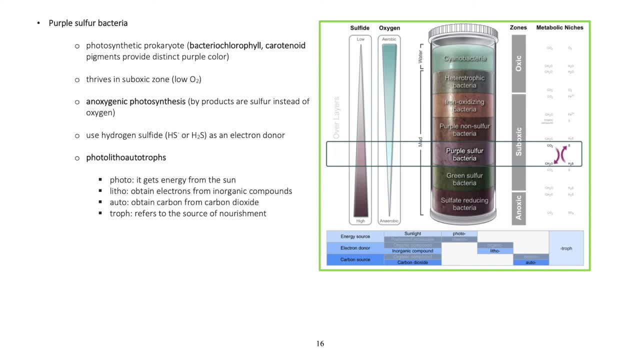 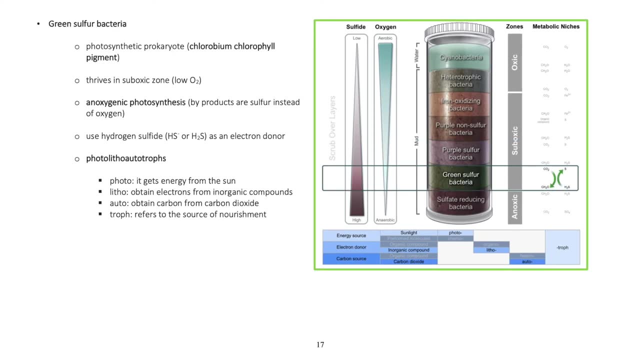 carbon dioxide And it gets energy from the sun. Polypropyl, And it's already 5,000我說 Photosynthetic prokaryotes, Presence of bacterioclorophyll And carotenoid pigments. Photographic bio gary. 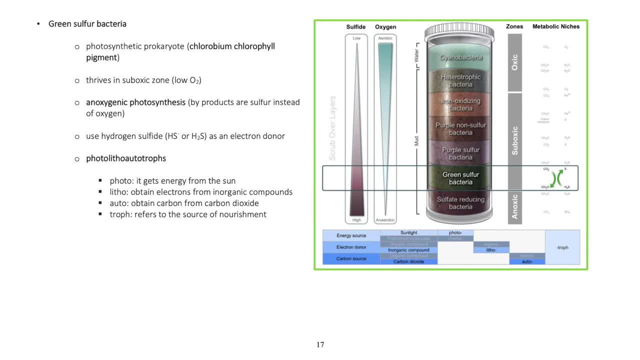 Photogenici, And it's already 5,000我說 Photogenici, And it's already 5,000. Said Troph Refers to the source of nourishment: green sulfur bacteria, Photosynthetic prokaryote, Presence of chlorobium, chlorophyll pigment. 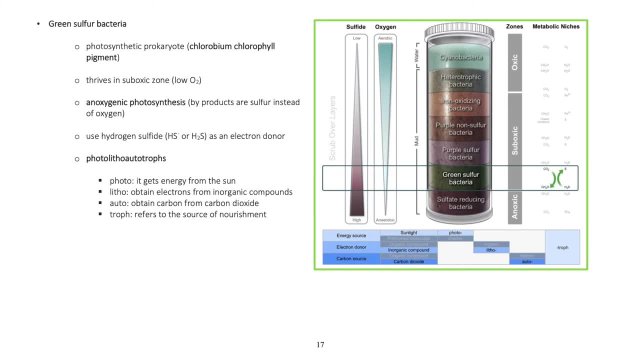 Thrives in suboxic zone. low oxygen Anoxygenic photosynthesis Byproducts are sulfur instead of oxygen. Use hydrogen sulfide as an electron donor. Photolithonidroph, And it's already 5,000 said Photogenic prokaryotes, And it's already 5,000 said Photarntoxic prokaryotes, And it's already. 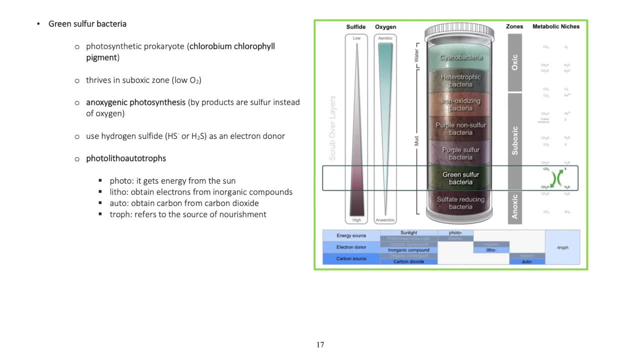 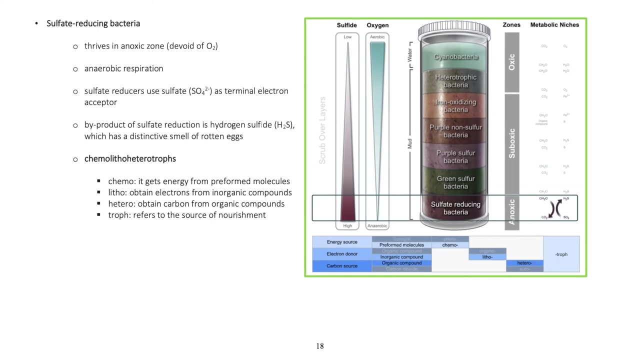 Photolithoautotrophs. Photo: It gets energy from the sun. Litho Obtain electrons from inorganic compounds. Auto Obtain carbon from carbon dioxide. Troph Refers to the source of nourishment. Sulfate-reducing bacteria Thrives in anoxic zone devoid of oxygen. Anaerobic respiration. 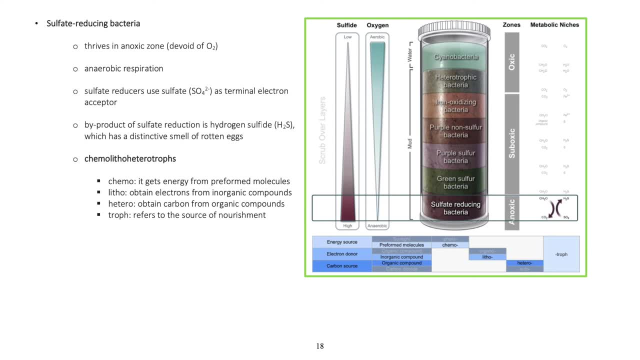 Fate-reducers use sulfate as terminal electron acceptor. Byproduct of sulfate reduction is hydrogen sulfide, which has a distinctive smell of rotten eggs. Chemolithoaneurotrophs, Chemo. It gets energy from preformed molecules. Litho Obtain electrons from inorganic compounds. 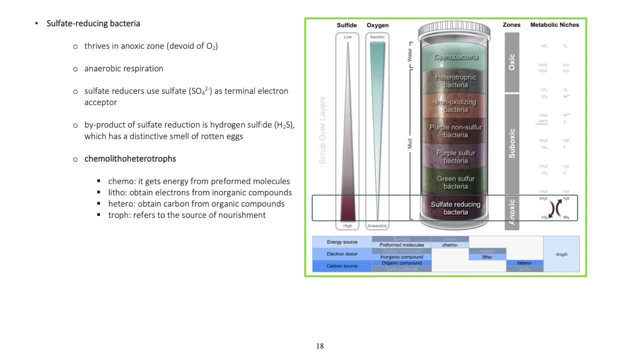 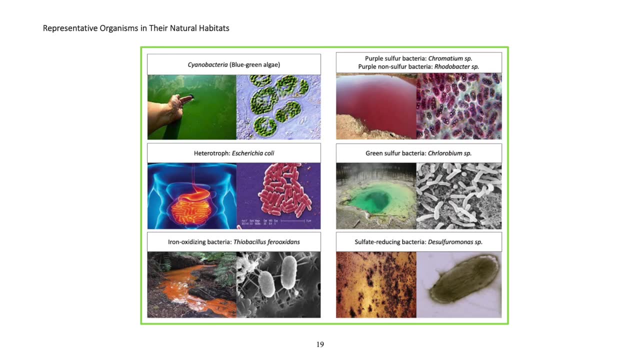 Haotero Obtain carbon from organic compounds. Troph Refers to the source of nourishment Representative organisms in their natural habitats: Cyanobacteria or blue-green algae. Haotero-troph- Acherichia coli- Iron-oxidizing bacteria. 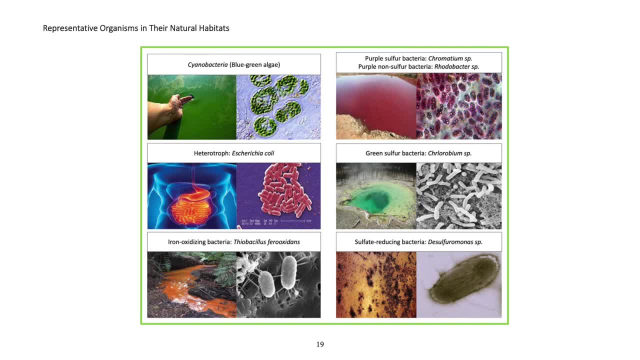 Theobacillus ferrooxidans. Purple sulfur bacteria. Chromadium sp. Purple non-sulfur bacteria. Rhodobacter sp. Green sulfur bacteria. Chlorobium sp. Sulfate-reducing bacteria. Desulfuromonas sp. 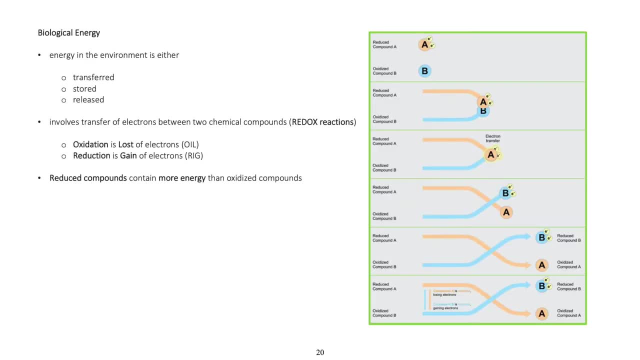 Biological energy. Energy in the environment is either transferred, stored or released. Involves transfer of electrons between two chemical compounds, Redox reactions. Oxidation is lost of electrons, Reduction is gain of electrons. Reduced compounds contain more energy than oxidized compounds. 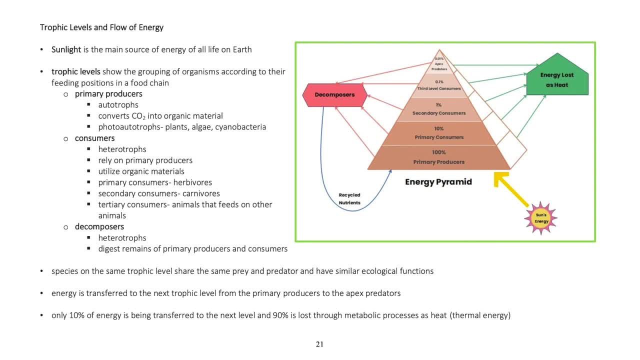 Chlorobacter. Electronic winter sources of oxygen, Trophic levels and flow of energy. Sunlight is the main source of energy of all life on Earth. Trophic levels show the grouping of organisms according to their feeding positions in a food chain. 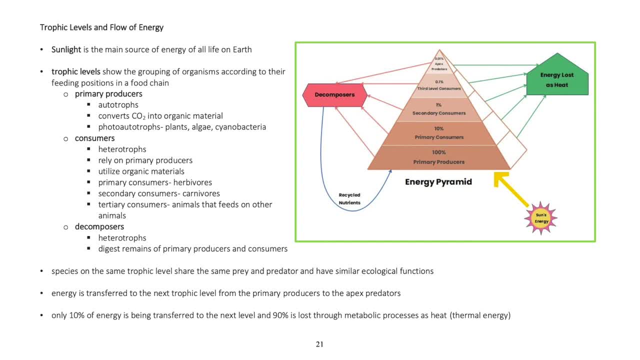 Primary producers. Autotrophs Converts carbon dioxide into organic material. Photautotrophs: Plants, algae, cyanobacteria. Paleontologists are the culprits. Plants, algae, cyanobacteria, bacteria Consumers. Heterotrophs: Rely on primary producers. Utilize organic